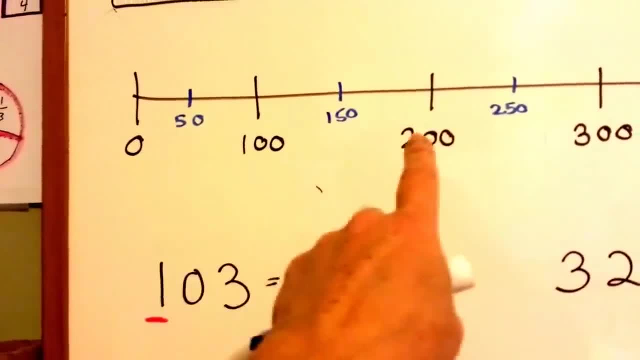 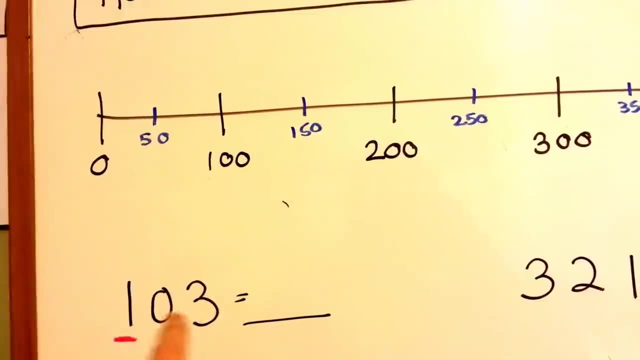 103.. Where would 103 go? Where would 103 be here? Would 103 be closer to 100 or 200?? Well, 103 would be very, very close to 100, right here. and do you know how? I know? 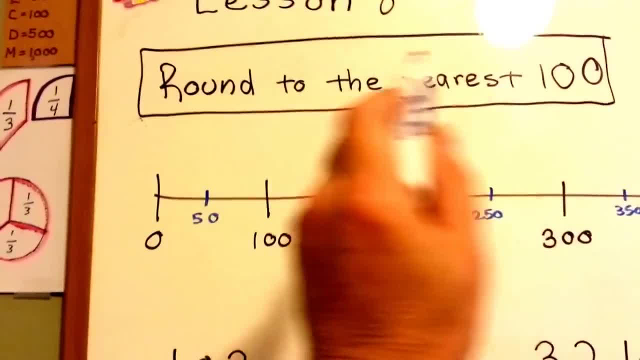 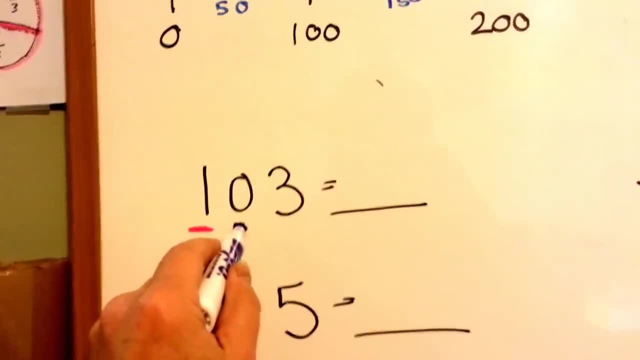 Because this is the 100's place. we're rounding to the nearest 100, the 1 is in the 100's place, so the 1 to the right of it. this one is telling it what to do, and I know that a 0 tells it to stay the same. 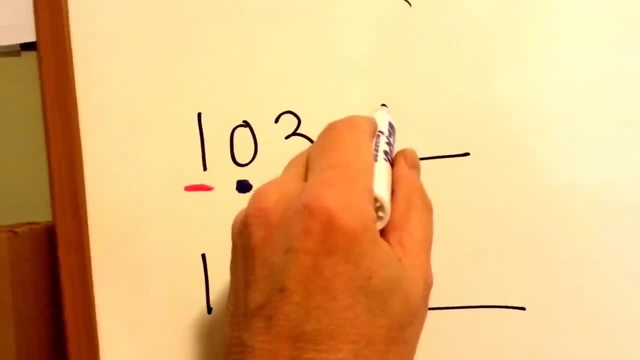 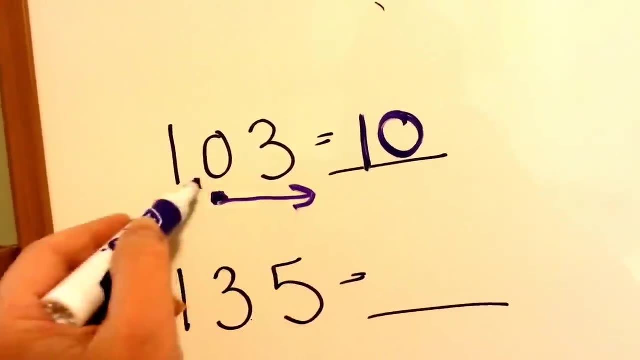 It's telling the 1.. It's telling the 1 to stay the same. Now that it's done with its job, it turns into a 0, and any number to the right of it also turns into a 0. It says, hey, I'm turning into a 0,, you turn into a 0 too. 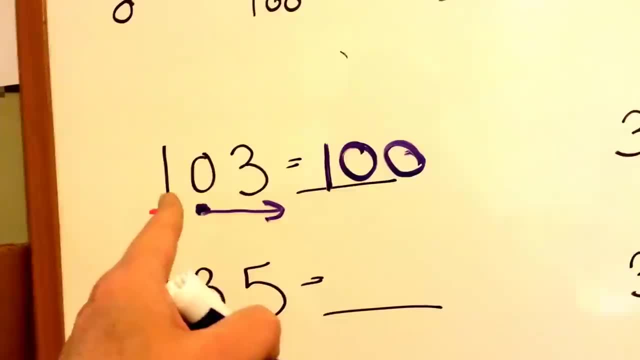 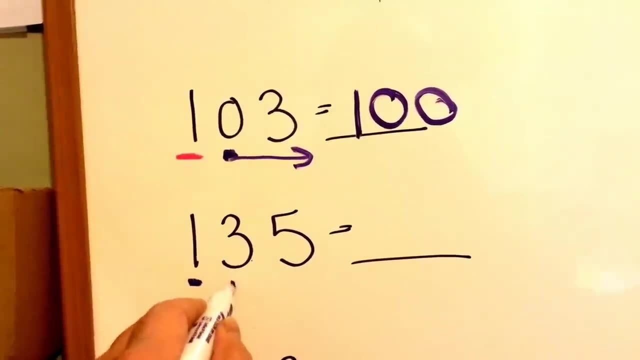 Also, So these both turn into a 0, and the 1 stays the same. What about 135?? This is the number we're rounding to, and the 3 tells it what to do. So the 3 tells it what to do. 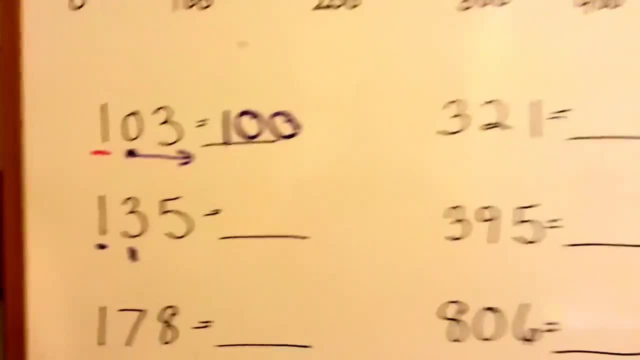 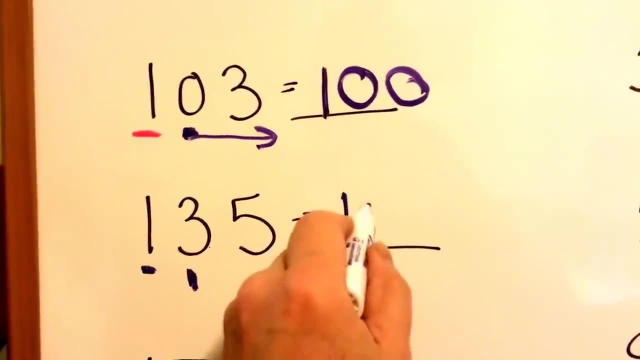 The 3 tells the 1 to stay the same. He says hey, 1, stay the same. And 1 says okay. 3 says I'm done doing my job, I'm turning into a 0.. Hey, Mr 5,, you turn into a 0 also. 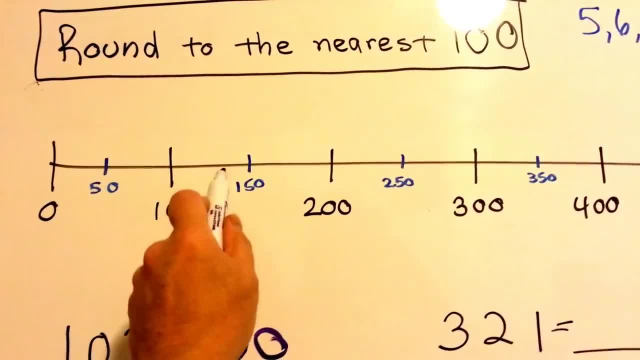 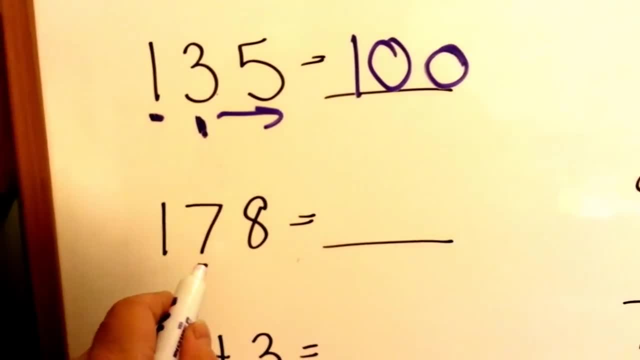 So 135,, which would be about right here, is closer to 100 than it is to 200.. See that. What about 178?? What is the 7 telling the 1 to do? Should it stay the same or should it go bigger? 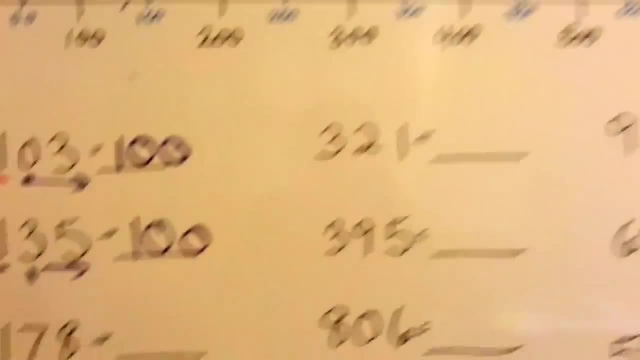 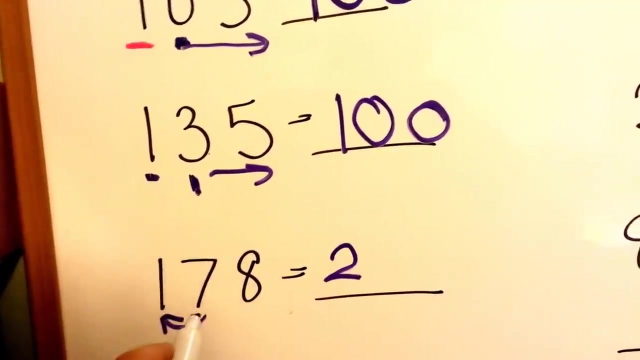 Well, a 7 tells it to go bigger. 7 says to the 1, you have to go bigger. to a 2,, the next biggest number. So he does, And 7 says: I'm done doing my job, I turn into a 0, and so does the 8.. 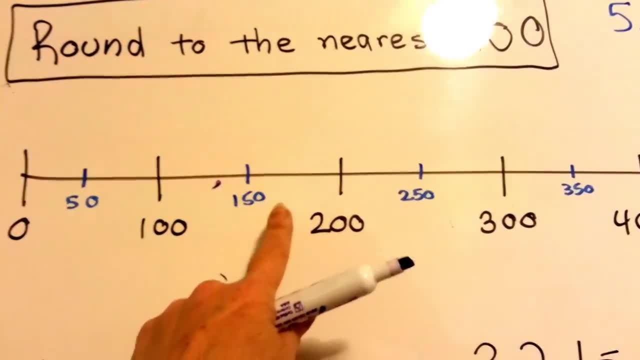 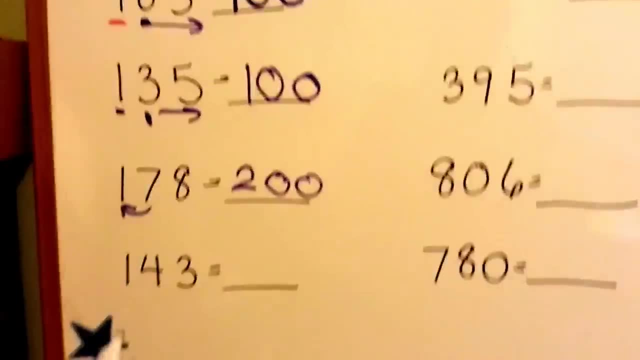 So 178, it's bigger than 150,, it would be about right here- is closer to 200 than 100. Because it would be about right here. see How. about 143?? What does the 4 tell the 1 to do? 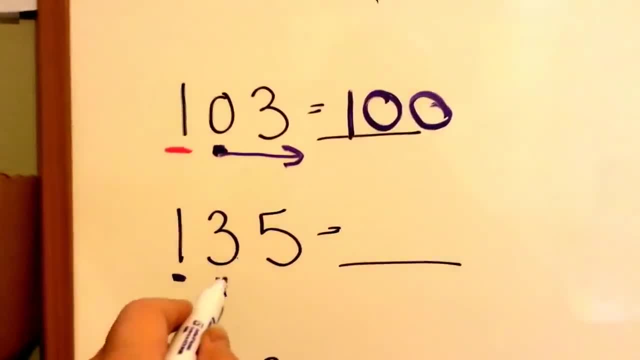 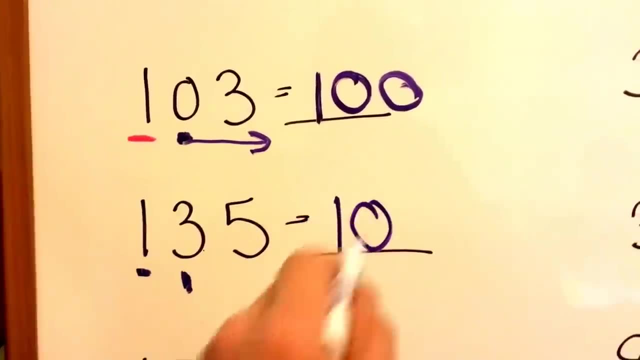 tells the one to stay the same, He says hey, one, stay the same. And one says okay. Three says I'm done doing my job, I'm turning into a zero. Hey, Mr Five, you turn into a zero also. So 135,. 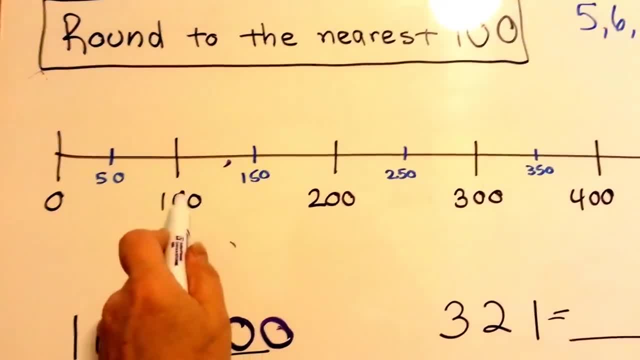 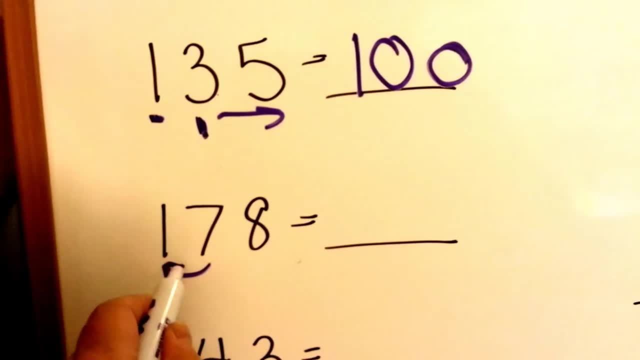 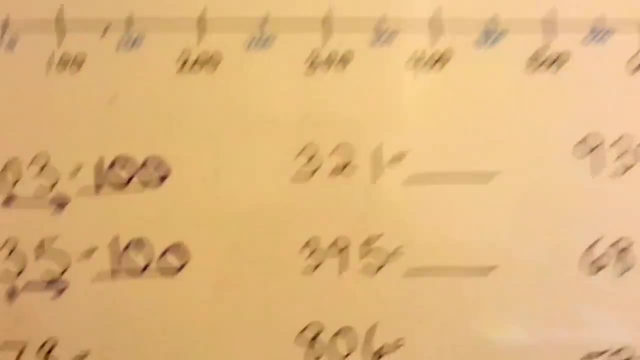 which would be about right here, is closer to 100 than it is to 200. See that. What about 178?? What is the seven telling the one to do? Should it stay the same or should it go bigger? Well, a seven tells it to go bigger. Seven says to the one: you have to go bigger. to a two: 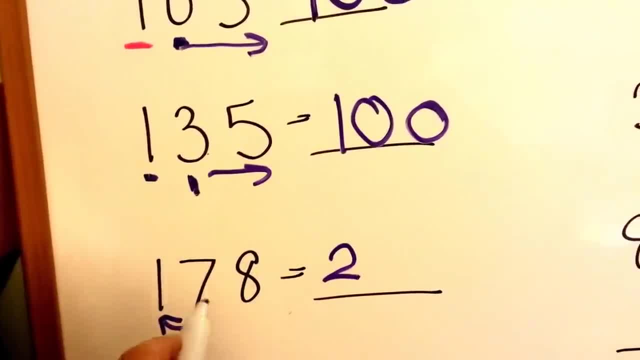 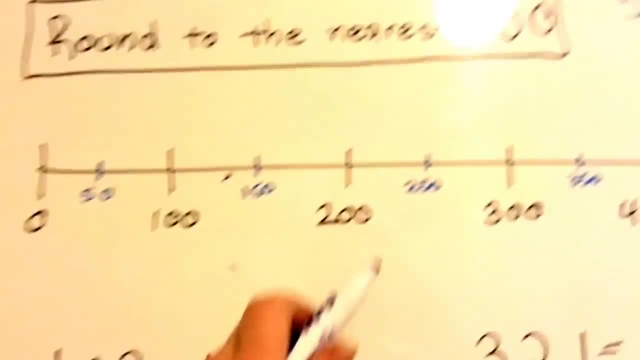 the next biggest number. So he does. And seven says: I'm done doing my job. I turn into a zero, and so does the eight. So 178, it's bigger than 150.. It would be about right here It's closer to 200 than 100.. 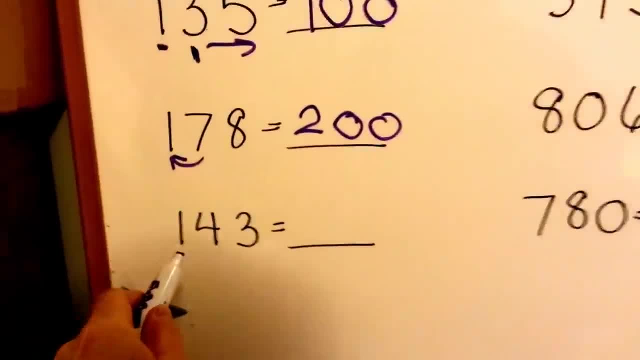 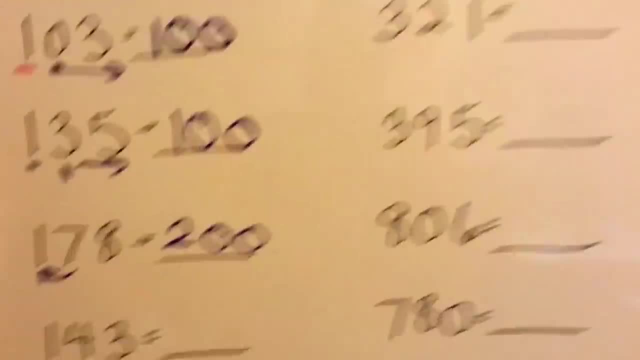 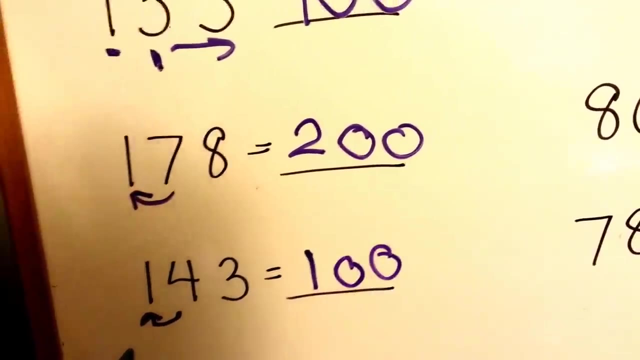 Because it would be about right here. See How, about 143?? What does the four tell the one to do? Remember, a four tells it to stay the same, So the one says, okay, I'm staying the same, And the four and the three are done and they turn into zeros. So 143 is closer to 100 than it is to. 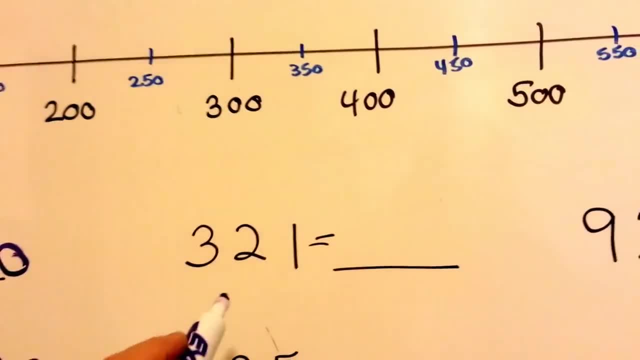 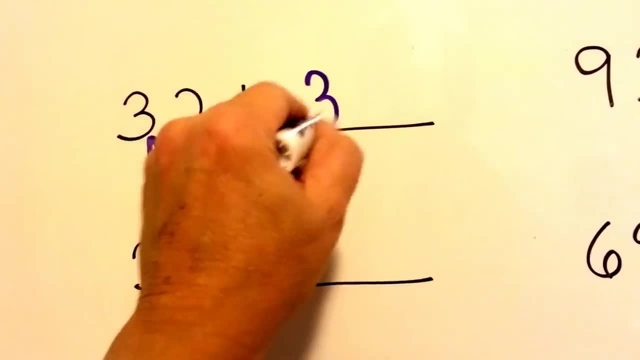 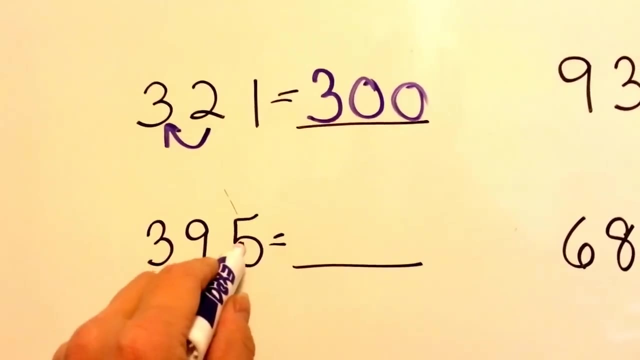 200.. What about 321?? The two tells it to stay the same. It's telling the three to go bigger. The three tells it to stay the same. So three is still a three. They're done doing their job and they turn into zeros. How about 395?? Well, the nine is the next one to the right, So it's the. 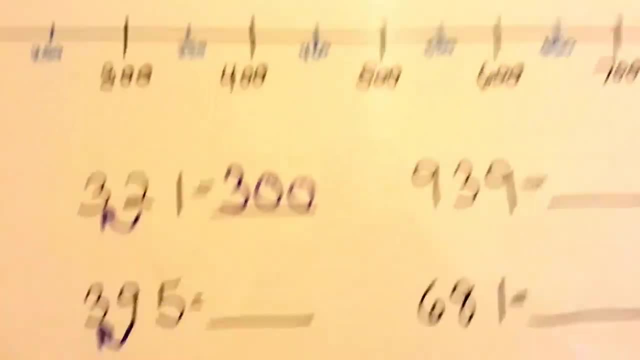 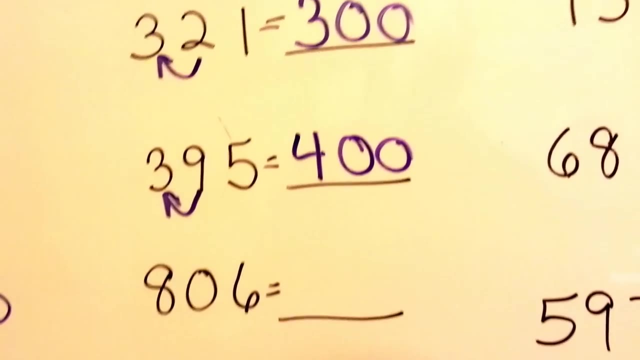 one telling it what to do And the nine tells it to go to the next biggest number. So the three is going to become a four. They're done doing their job and they turn into zeros. So 395 is closer to 400 than it is to 300.. 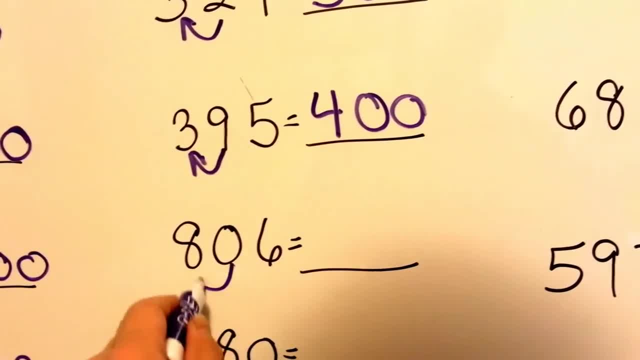 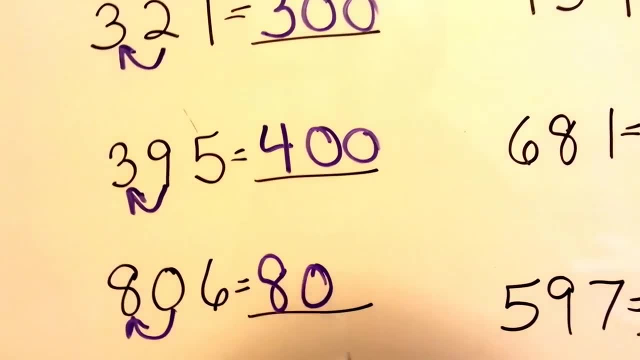 How about 806?? What does the zero tell the eight to do? Yeah, it tells it to stay the same. So eight is going to stay the same. Zero is zero. And it tells the six to be a zero. So 806 is closer to. 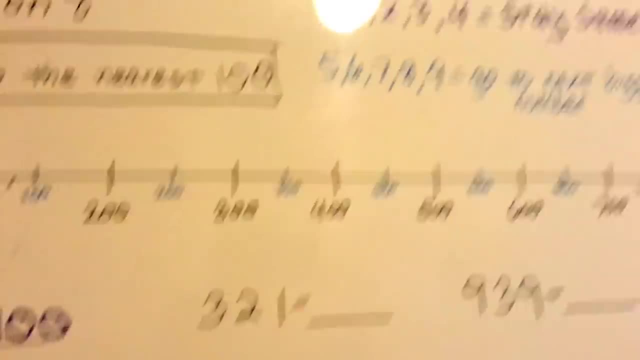 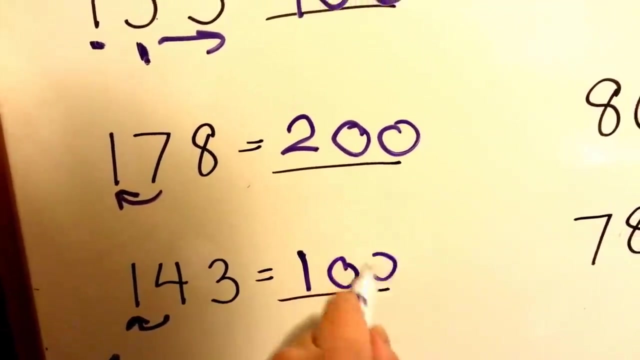 Remember: a 4 tells it to stay the same. So the 1 says, okay, I'm staying the same, And the 4 and the 3 are done and they turn into 0s. So 143 is closer to 100 than it is to 200. 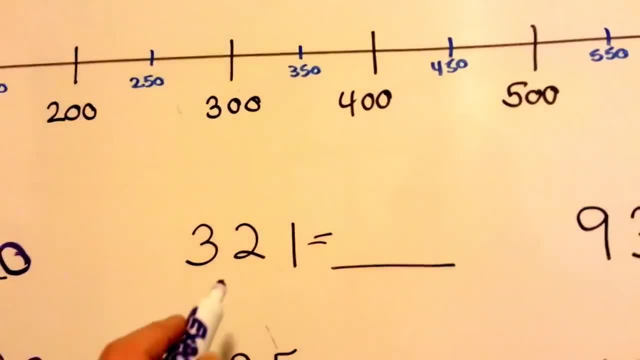 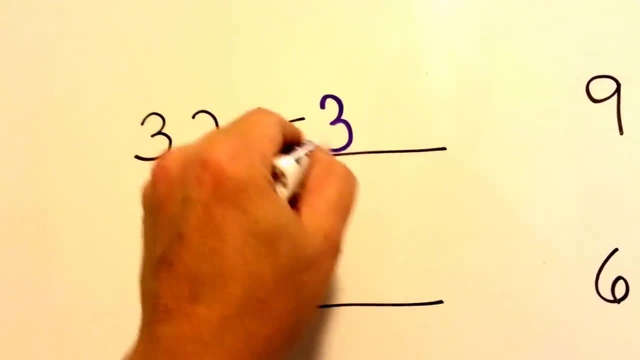 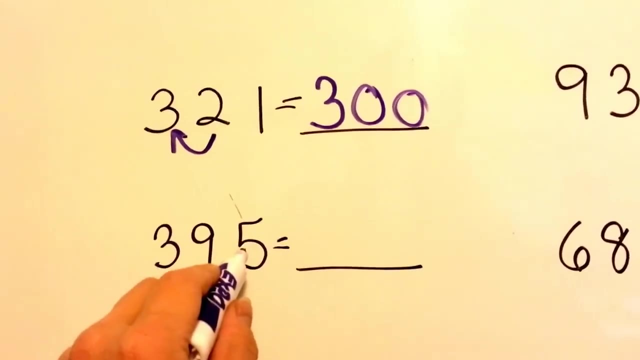 What about 321?? The 2 tells it to stay the same. It's telling the 3 to stay the same, So 3 is still a 3.. They're done doing their job and they turn into 0s. How about 395?? 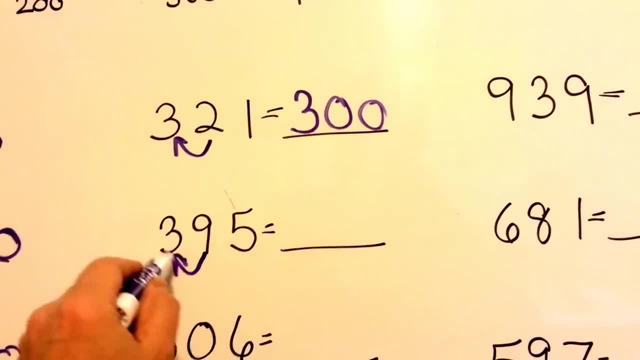 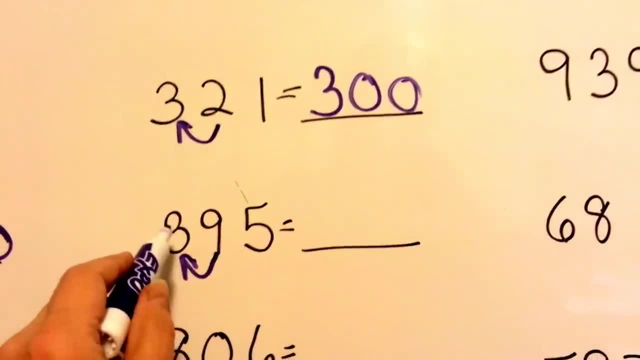 Well, the 9 is the next one to the right, so it's the one telling it what to do, and the 9 tells it to go to the next biggest number. So the 3 is going to become a 4.. They're done doing their job and they turn into 0s. 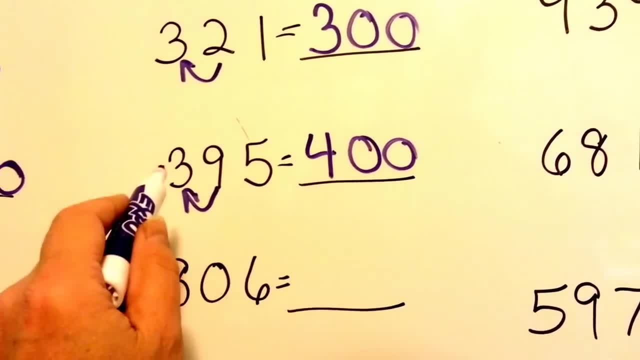 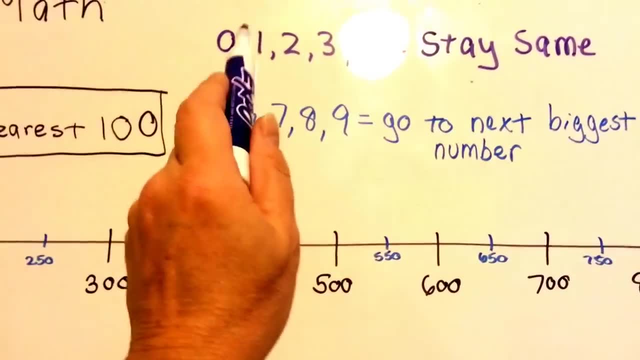 So 395 is closer to 400 than it is to 300.. How about 806?? What does the 0 tell the 8 to do? Yeah, it tells it to stay the same. So 8 is going to stay the same. 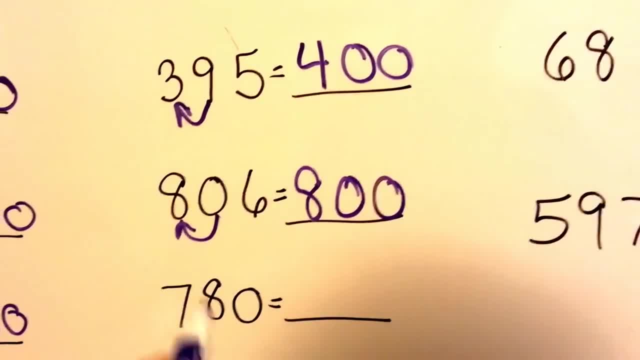 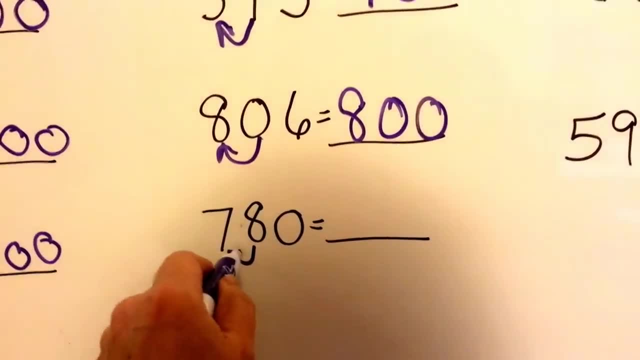 0 is 0, and it tells the 6 to be a 0.. So 806 is closer to 800 than it is to 900.. How about 780?? The 8 tells the 7 to go to the next biggest number. 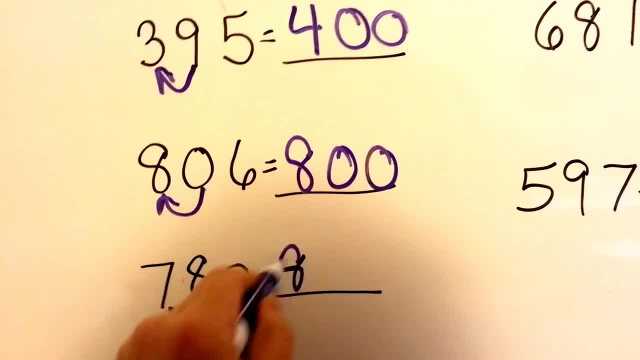 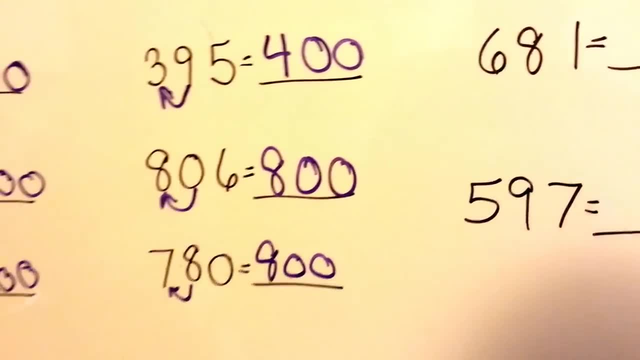 It's in the blue group right. So the 7 is going to become an 8, and these guys are 0s now because of the 8., Because they're finished doing their job, even though he kind of stayed a 0,, and so did he. 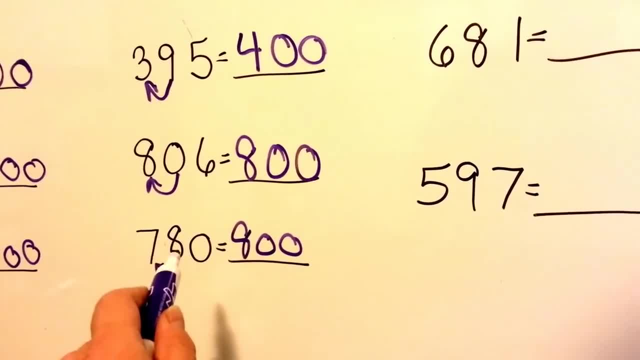 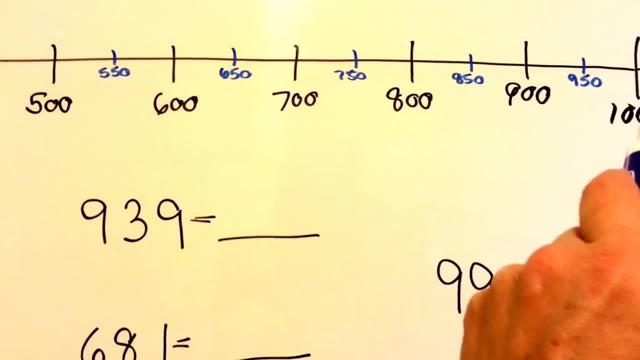 So 780 is closer to 800 than it is to 700.. What about 939?? 939, is it closer to 900 or 1,000?? The 3 is going to tell the 9 what to do. It's going to tell it to stay the same. 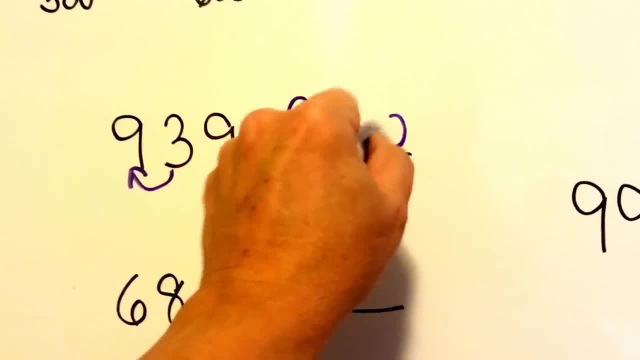 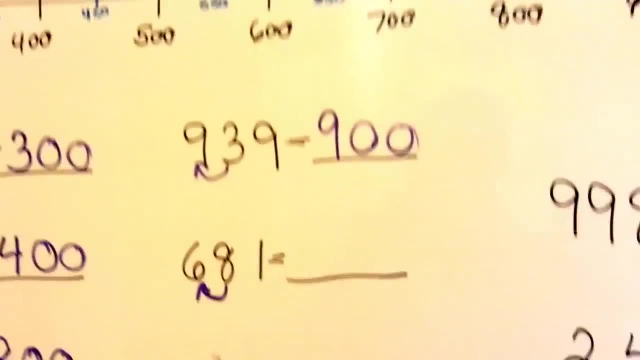 So 9 stays the same and these two guys turn into 0s. How about 681?? The 8 tells the 6 to go to the next biggest number. So 6 becomes a 7, and they become 0s. 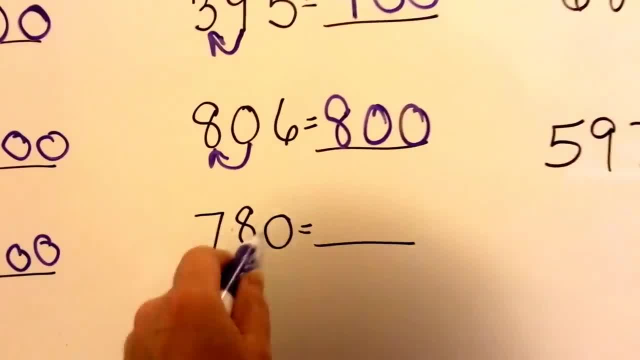 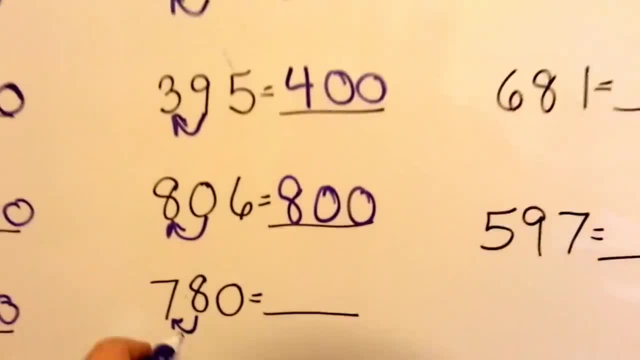 800 than it is to 900.. How about 780?? The eight tells the seven to go to the next biggest number. It's in the blue group, right? So the seven is going to become an eight, And these guys are done doing their job. 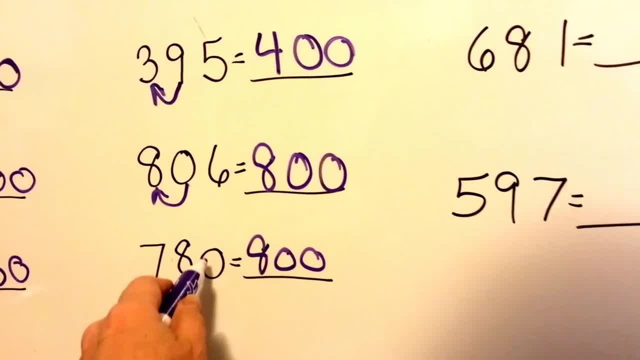 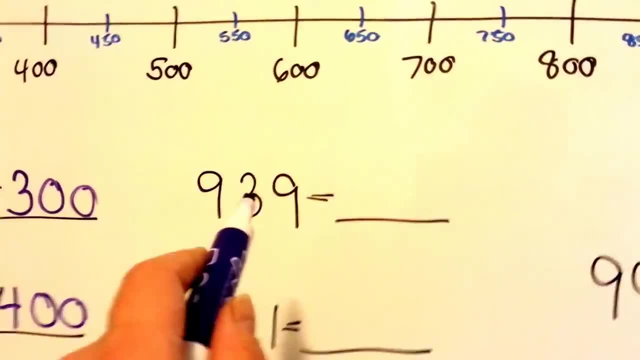 Now the nine and the eight are zeros now because they're finished doing their job, even though he kind of stayed a zero, and so did he. So 780 is closer to 800 than it is to 700.. What about 939?? 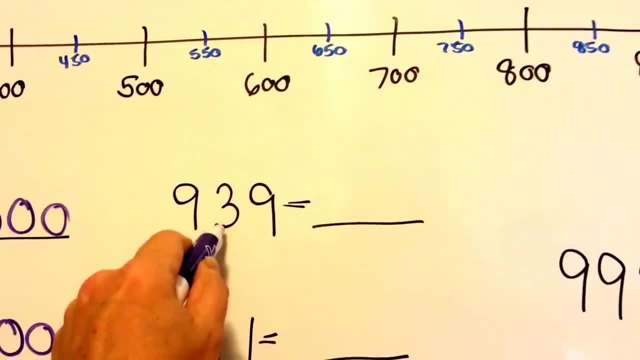 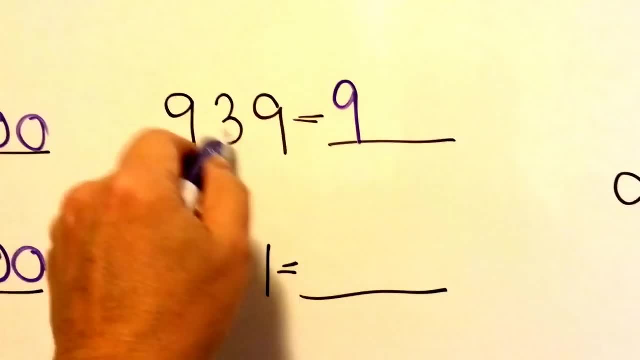 939. is it closer to 900 or 1000?? The three is going to tell the nine what to do. It's going to tell it to stay the same. So nine stays the same And these two guys turn into zeros. How about? 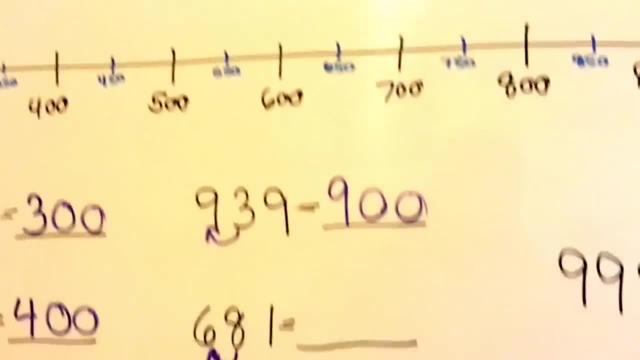 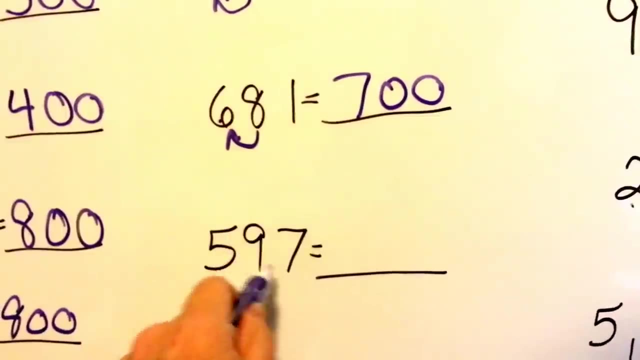 681?. The 8 tells the 6 to go to the next biggest number. So 6 becomes a 7, and they become zeros. A couple more: 597.. Is it closer to 500 or 600?? Yeah, it's closer to 600.. 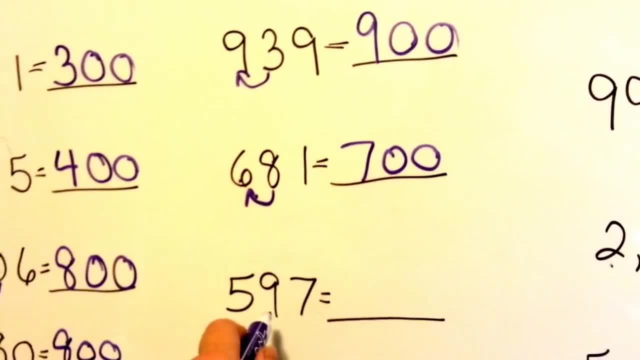 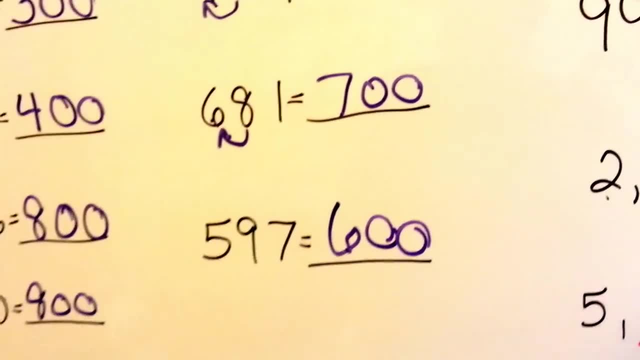 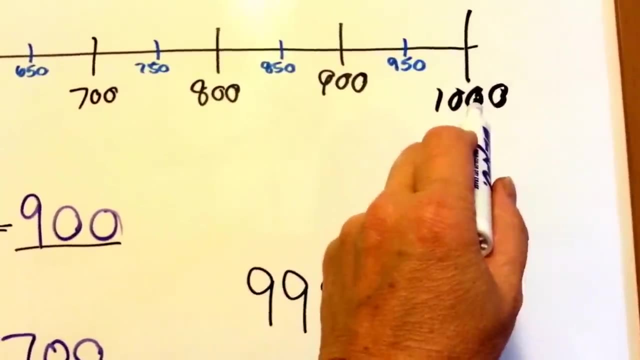 Just by a few digits, right, Just three more. The 9 tells the 5 to become a 6. And then it and the 7 have done their job and they become zeros. What about 998?? Is it closer to 900 or 1,000?? 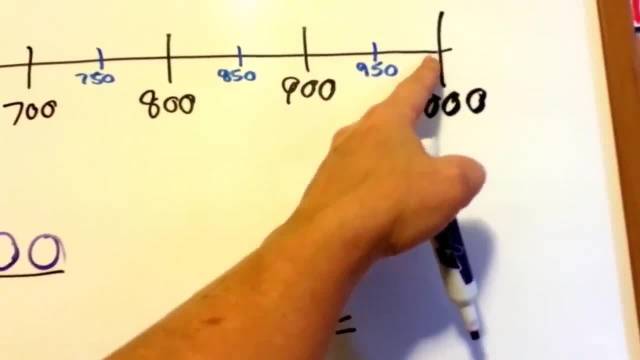 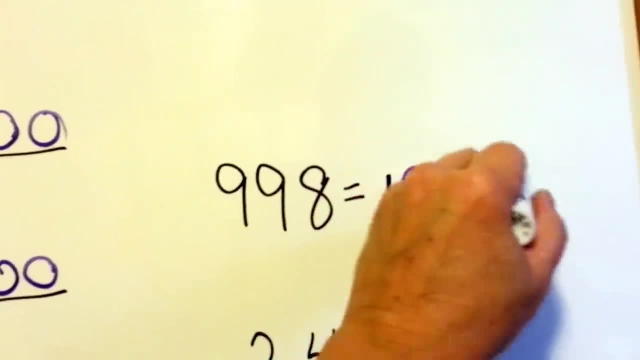 Wouldn't 998 be like right here, just a couple numbers away from 1,000? 998,, 999,, 1,000.. Yeah, So, even though we're rounding to the nearest hundred, this 9 tells that 9 to go up to the next number. 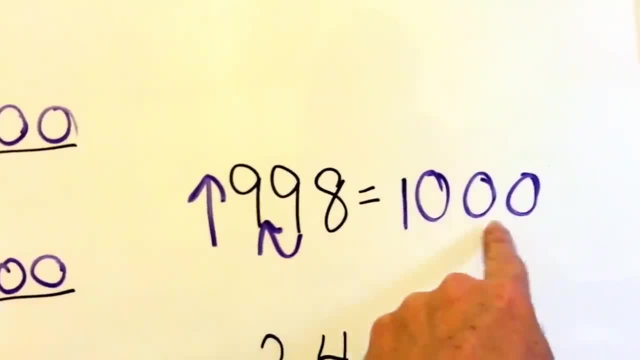 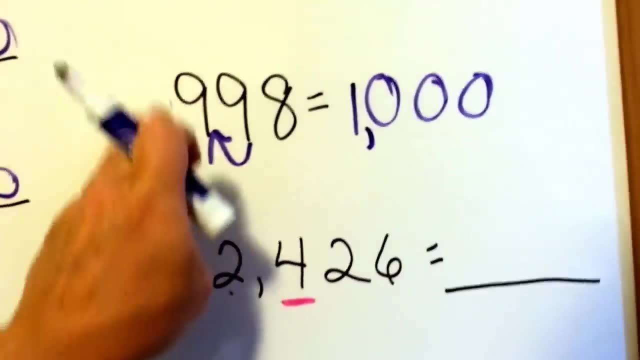 So the 9 goes up to a 10, and the 9 and the 8 become zeros. See, So it becomes 1,000.. So, yes, Even though we're rounding to the nearest hundred, you can round 998 to 1,000.. 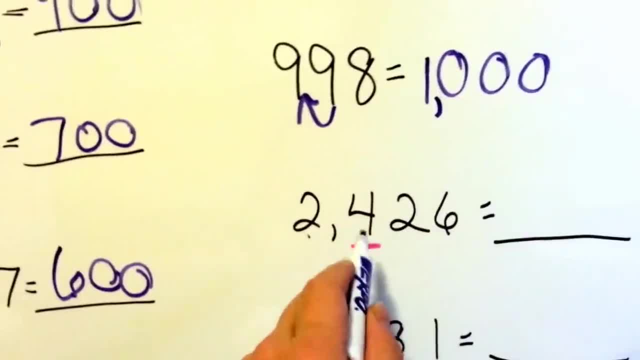 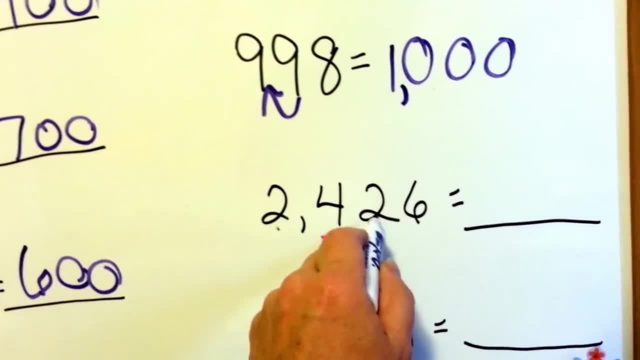 What if there's other numbers here? Now we're rounding to the hundred and the pink one is the hundred's place. You ignore this one until we're done. The 2 tells the 4 to do what. 2 tells it to stay the same. 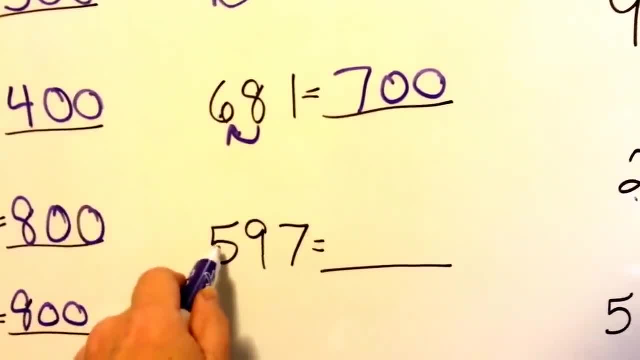 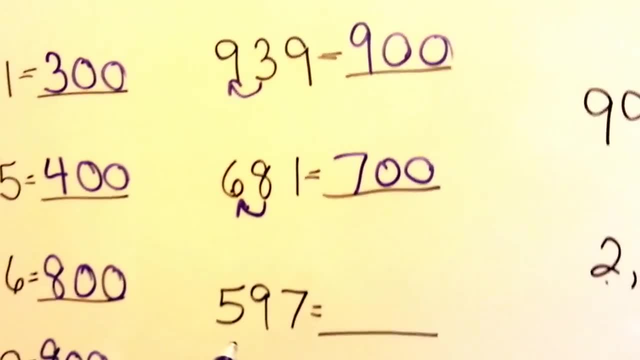 A couple more. 597, is it closer to 500 or 600?? Yeah, it's closer to 600, just by a few digits. right, Just three more. The 9 tells the 5 to become a 6,. 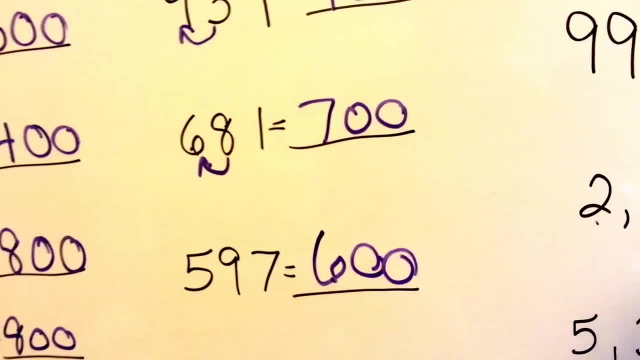 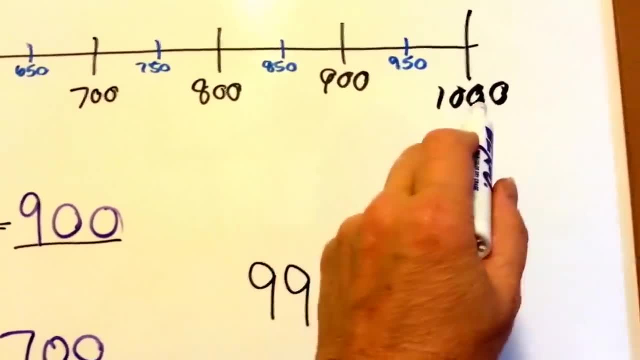 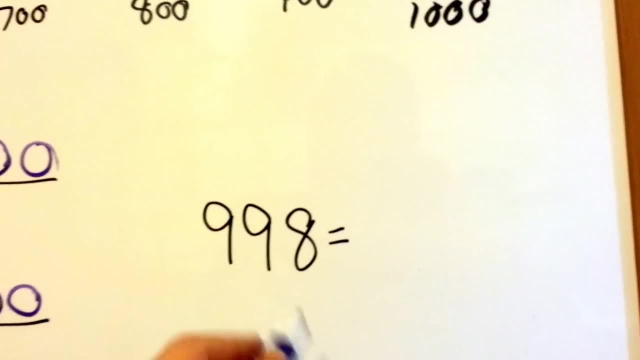 and then it and the 7 have done their job and they become 0s. What about 900?? What about 998?? Is it closer to 900 or 1,000?? Wouldn't 998 be like right here, just a couple numbers away from 1,000?? 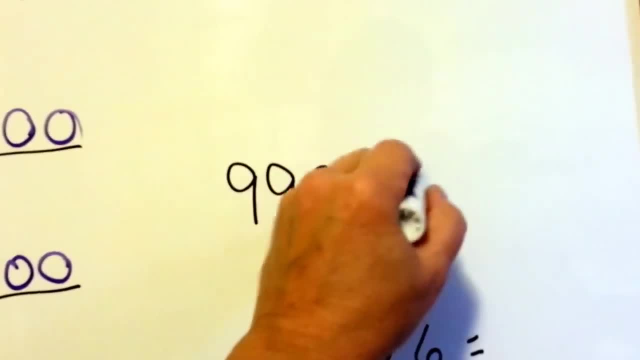 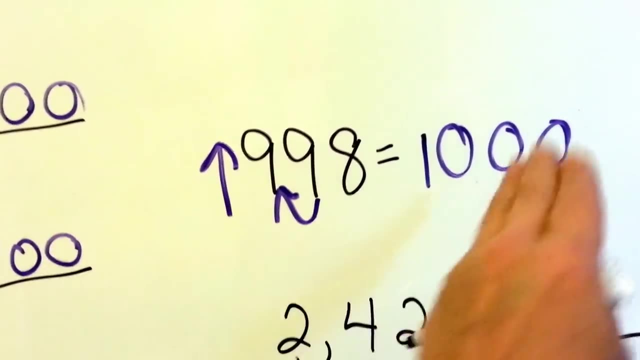 998,, 999,, 1,000.. Yeah, So, even though we're rounding to the nearest 100, this 9 tells that 9 to go up to the next number. So the 9 goes up to a 10,. 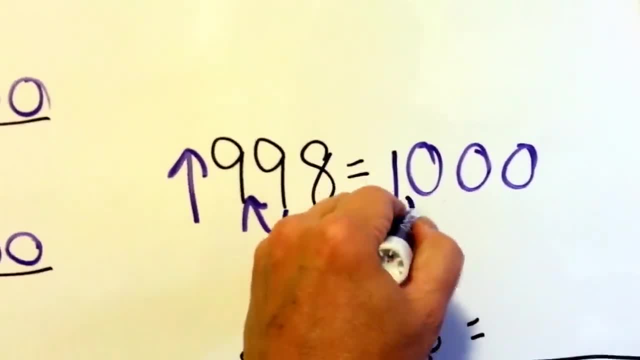 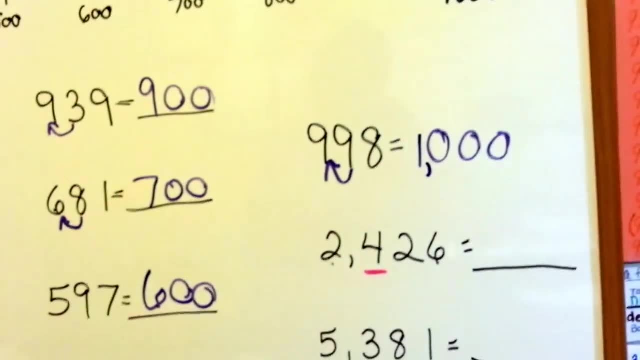 and the 9 and the 8 become 0s. see, So it becomes 1,000.. So, yes, even though we're rounding to the nearest 100, you can round 998 to 1,000.. What if there's other numbers here? 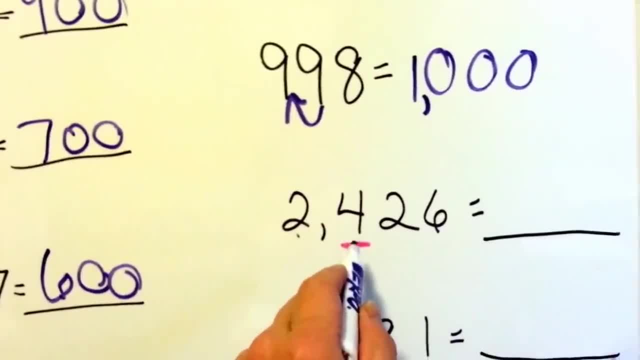 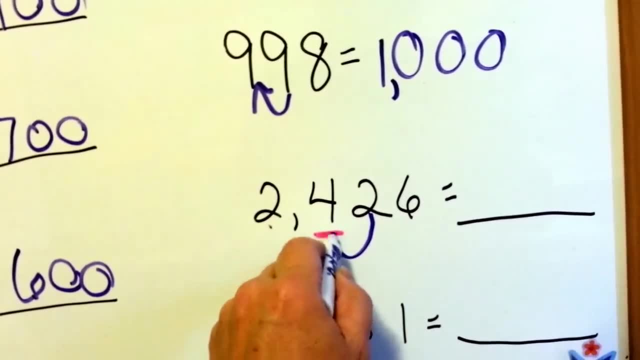 Now we're rounding to the 100, and the pink one is the 100's place. You ignore this one until we're done. The 2 tells the 4 to do what 2 tells it to stay the same. So the 4 is going to stay the same. 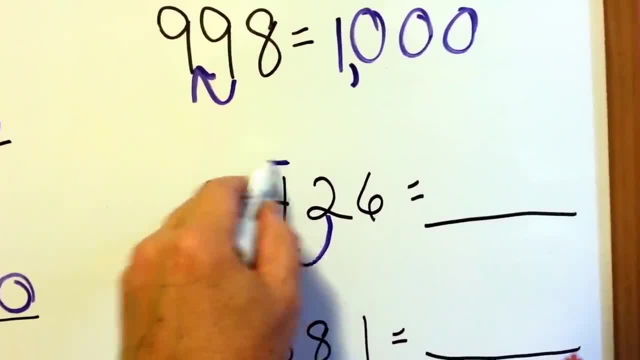 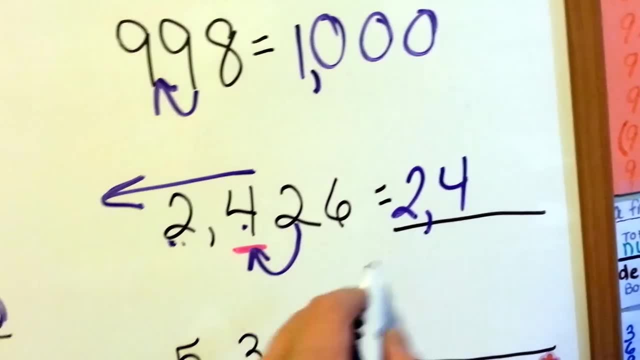 He has to bring him along. Anybody that is on this side is just going to go for the ride, So the 2 is going for the ride, 4 is staying the same, And the 2 and the 6 are finished doing their job. 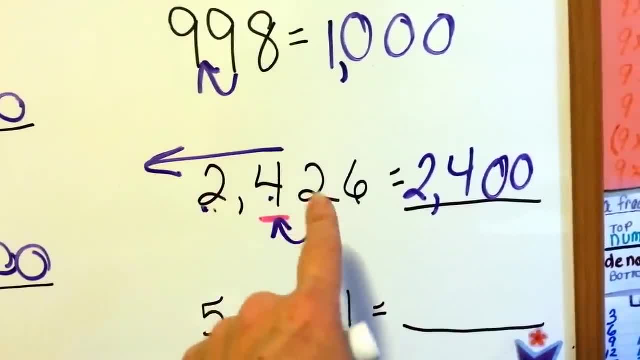 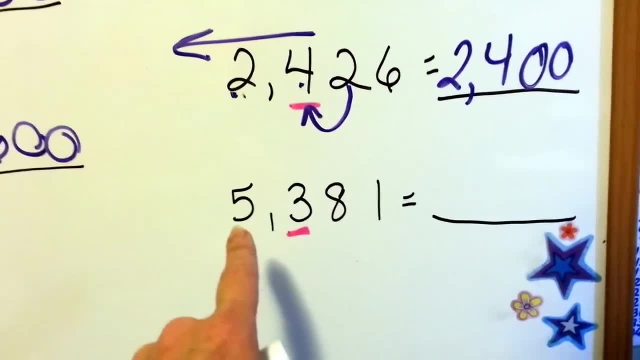 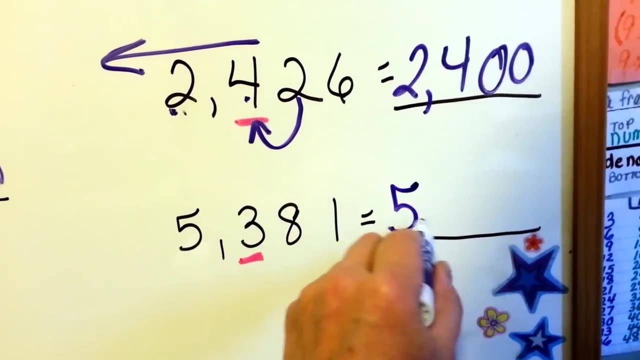 They turn into 0s. So 2,426 rounded to the nearest 100 becomes 2,400.. What about this one, 5,381?? Well, the 5 is just going to go for the ride. Let's just put them here. 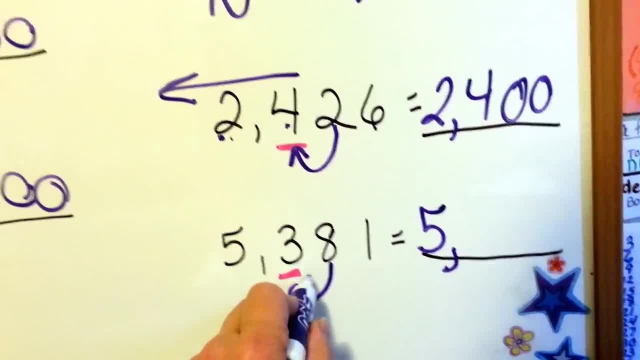 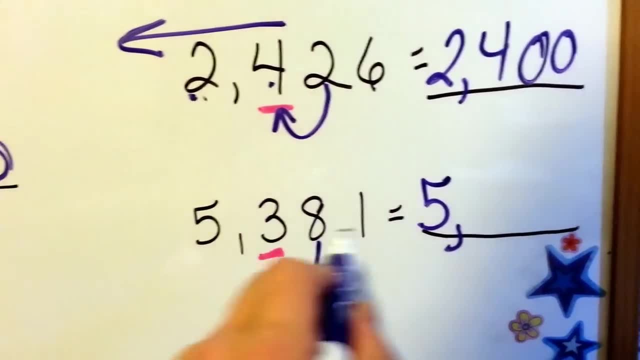 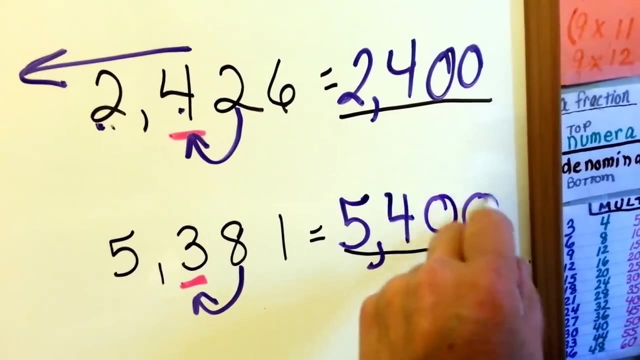 And the 8 tells the 3 to go up to the biggest number, the bigger number. So 3 is going to become a 4. And the 8 and the 1 are finished doing their job and they become 0s.